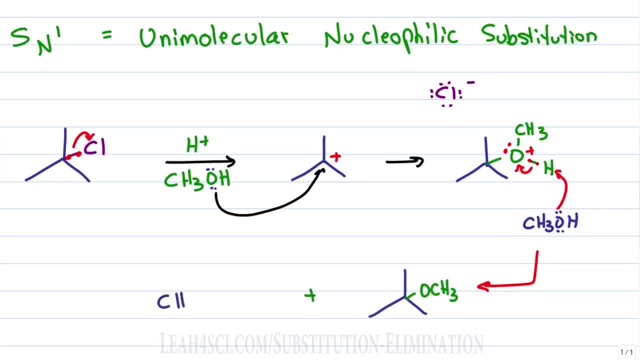 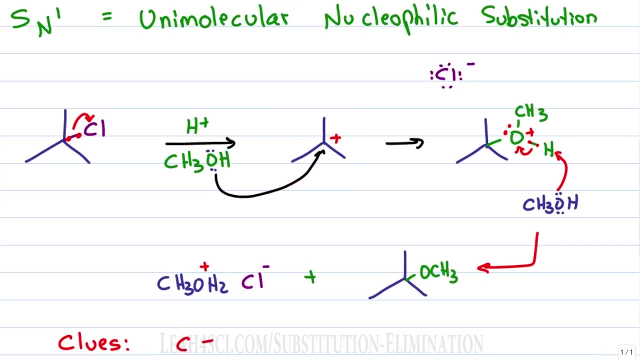 molecule as a CH3OH2+, with it's counter ion, the leaving group as Cl-. The clues to recognize that an SN1 reaction takes place is as follows: Carbocation intermediate as the rate determining slow step and a solvent nuclear file attached to the so-called NH5. 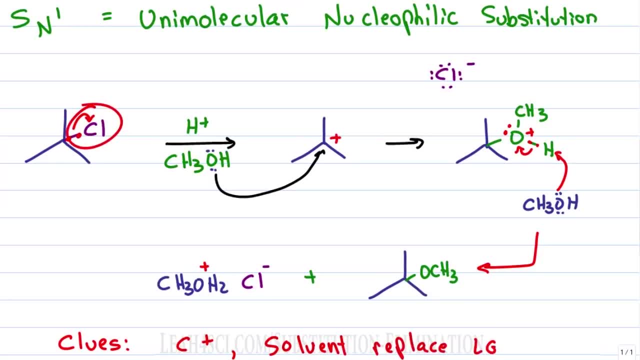 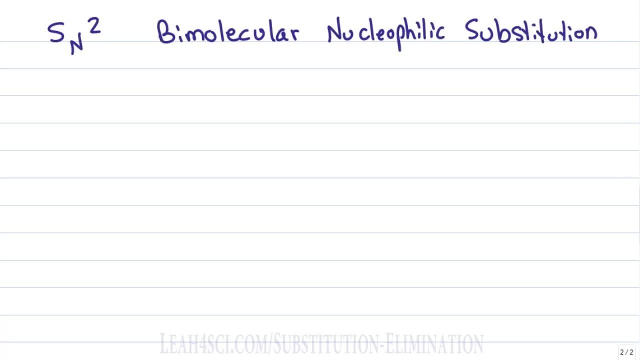 block where the leaving group used to be. SN2 stands for bimolecular nucleophilic substitution, where bimolecular is two molecules reacting at the same time in a one step, no intermediate reaction. For this reaction we have a primary leaving group reacting with NASH in a polar aprotic solvent. 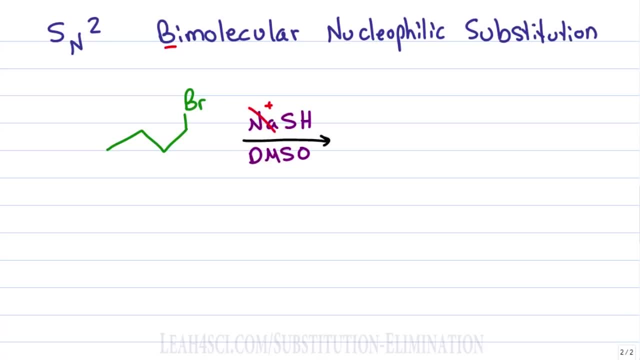 DMSO. Anytime you see, NA recognize the spectator positive ion to give us a negative S, which is a good nucleophile. This is a fast reaction because we're not waiting for a carbocation to form. Instead, the nucleophile will take its low in electrons, directly attack the carbon holding. 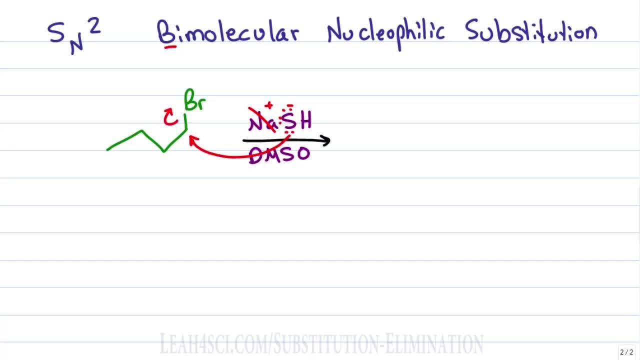 the leaving group to kick that out so that in one single step we get the entire product. SH is now attached where bromine leaving group used to be and the leaving group is floating in the carbon holding. the leaving group SH is floating around somewhere in solution. This product is achiral, but in the case of a chiral, 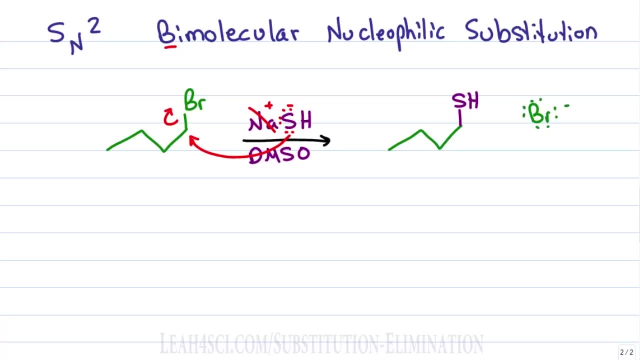 starting molecule, you would get an inversion of the initial configuration for SN2 reactions. The clues for this reaction are as follows: We have absolutely no carbocation intermediate. This is a fast reaction that happens in one step, and the fact that the nucleophile sits on the carbon, where the leaving group used to be. 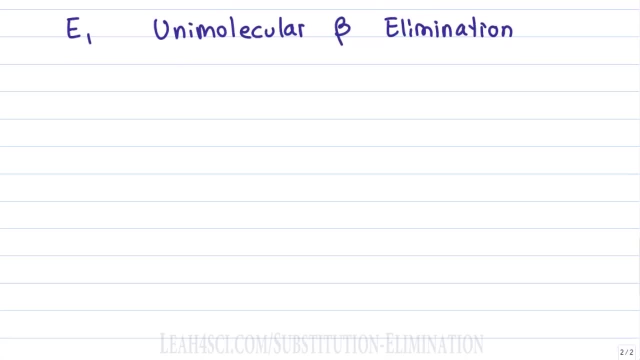 SH is floating around somewhere in solution. This product is achiral, but in the case of a chiral starting molecule you would get an inversion of the initial configuration. for SN2 reactions, E1 stands for unimolecular beta elimination. This is similar to the SN1 reaction and is often in 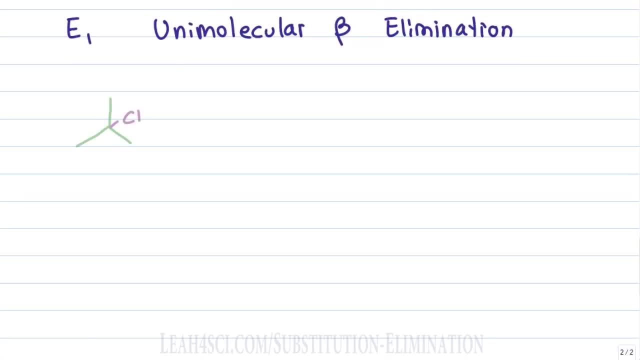 competition. In fact, we'll demonstrate this reaction using the same starting molecule and reagent. The only difference is that we'll add heat, because this will help us favor elimination over substitution. The mechanism begins in the same way, where the leaving group will grab the electrons binding it to carbon and break away to give us a carbocation. 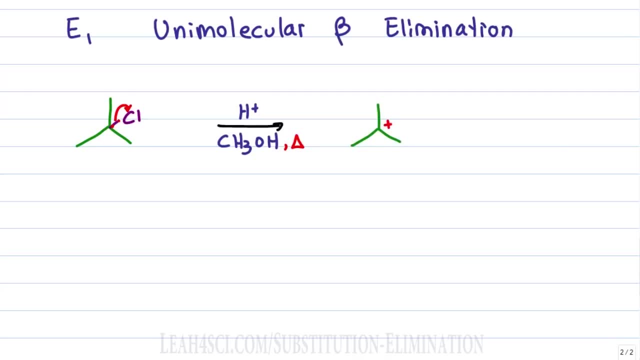 This is the rate determining slow step of the reaction, where the leaving group just wanders away somewhere in solution For elimination. instead of a solvolysis, where the nucleophile attacks the carbocation directly, the nucleophile is looking for a beta hydrogen, a hydrogen that 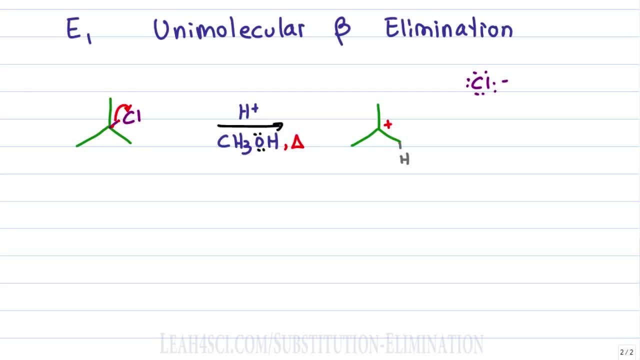 sits on the carbon next to the carbocation and it'll use its electrons to pluck off that hydrogen. The electrons that bind hydrogen to carbon will stay on the molecule and collect the carbon and collapse towards the positive charge to give us our final product, which has a pi bond between the 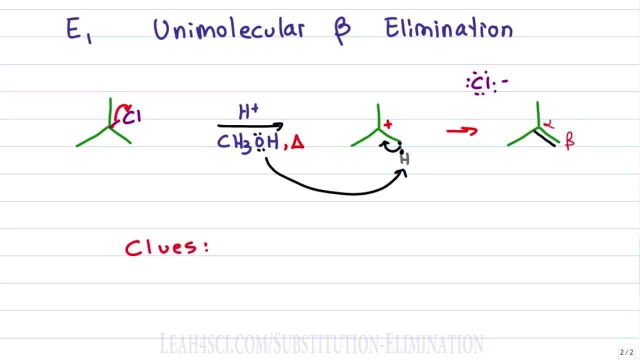 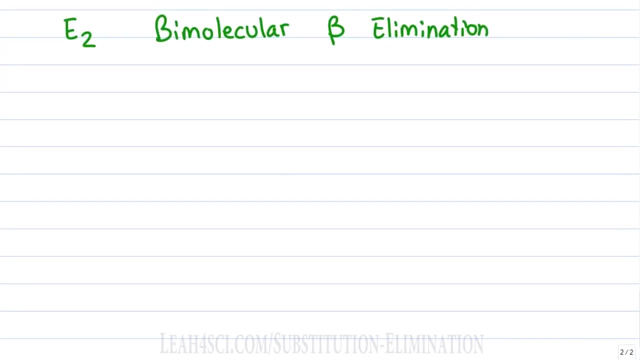 alpha and beta carbon. The clues that an E1 reaction took place is as follows: One, you have a carbocation intermediate and two, you have a pi bond between the alpha and beta carbon. E2 reaction is a bimolecular beta elimination. Bi tells us two molecules. 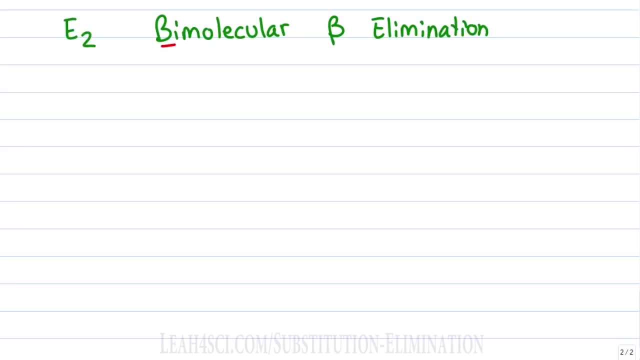 reacting at the same time. that means no intermediate for a fast one step reaction. For this E2 reaction, we'll look at a secondary leaving group reacting with NaOCH3 and CH3OH, recognizing that Na is a positive spectator, giving us a negative base, in this case CH3O-. 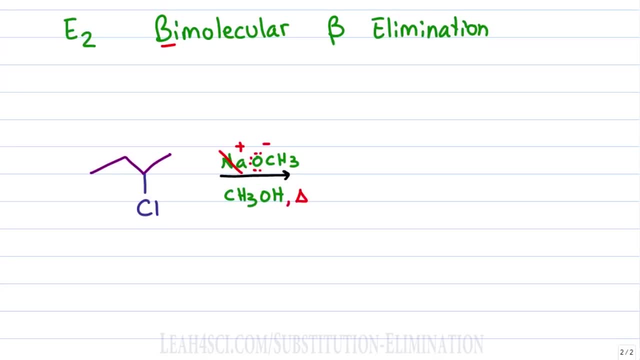 or methoxide. We'll add in heat to help stabilize the pi bond formation intermediates. This will favor an E2 over SN2 reaction, Like the E1 reaction. we're not attacking directly. instead we're looking for the most substituted beta hydrogen so that the base can grab the hydrogen and pull it off the molecule. 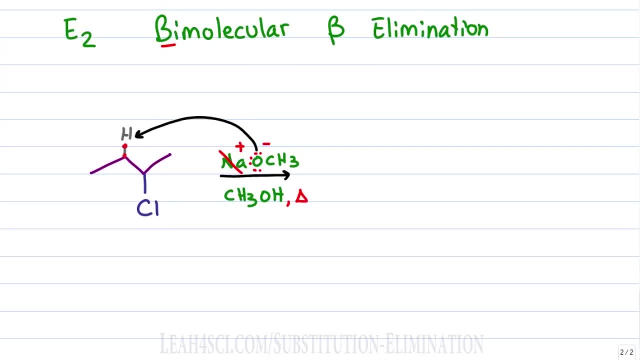 This will cause the electrons between hydrogen and the carbon to collapse in the direction of the leaving group, kicking out the leaving group, so that this is a one step, absolutely no intermediate reaction to give us the product. The product is a pi-bond between the alpha and more substituted beta carbon for the Zet-7. 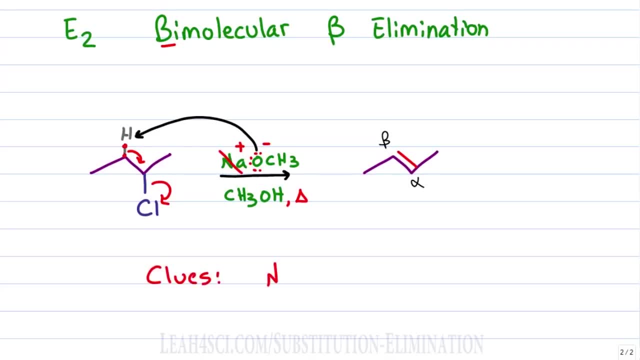 elimination. The clues that this reaction took place includes absolutely no carbocation intermediate, because we have a strong attacker and a fast one step reaction. Our second clue is a pi-bond between the alpha and more substituted beta carbon. Do you need to see these reactions in more detail?